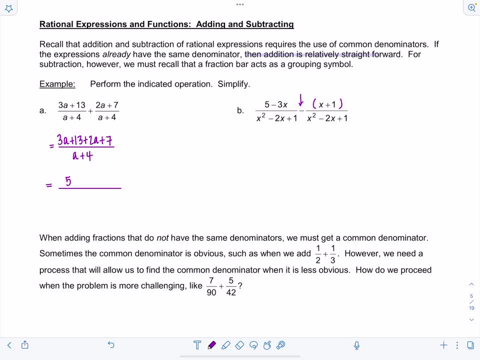 We've got 3a and 2a, So that's 5a, And then 13 plus 7, that's 20.. And we still have a plus 4 in the denominator. Okay now before you think, oh, we're done, let's box it. Always make sure. 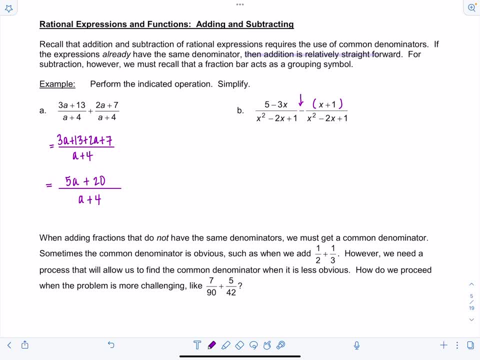 that your expression is completely simplified. So think back to the last video, when we only focused on simplifying rational expressions. we made sure that we factored the numerator denominator and canceled common factors. So be on the lookout. No one's going to remind you. 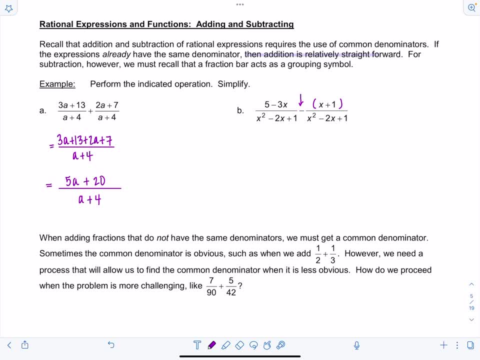 you got to remember to do that as your final step. And look at the numerator. here we've got 5a plus 20.. Can't I factor out a 5 from both those terms upstairs? Yep, I sure can. So this is 5 times a. 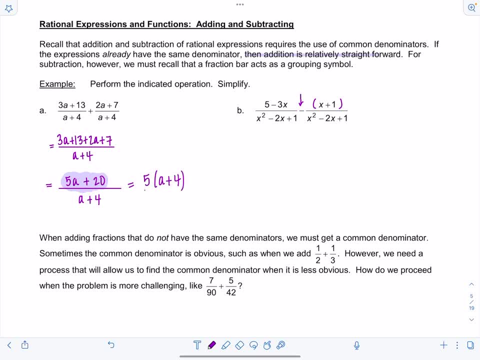 plus good 4 over a plus 4.. And notice, now a plus 4 is going to cancel out And I'm just left with 5.. Wow, wow, wow. Okay. so that's our final answer. How do you feel? A little scared, You're like I'm not going to. 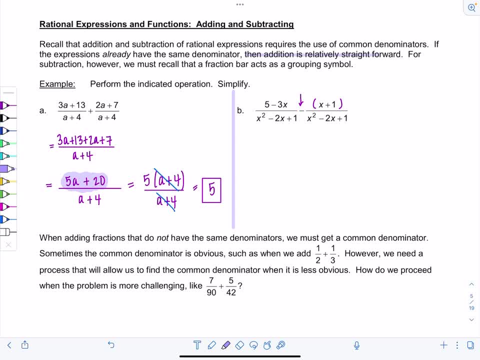 remember to factor at the end. Oh no, don't worry, We're just going to drill it into you So it'll become second nature. All right now notice in example B we have subtraction. So I made the point to remind you to put parentheses around all the terms in the numerator, if it helps you. 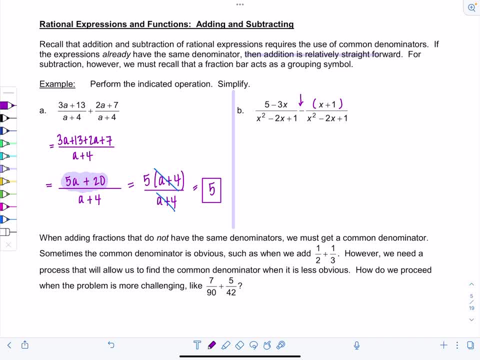 remember to distribute that negative. And again, we have a common denominator already, So I don't have to do anything with it. I say: rewrite the denominator first so you don't get carried away and do something weird. So don't change anything, leave the denominator as is. And now I'm going to 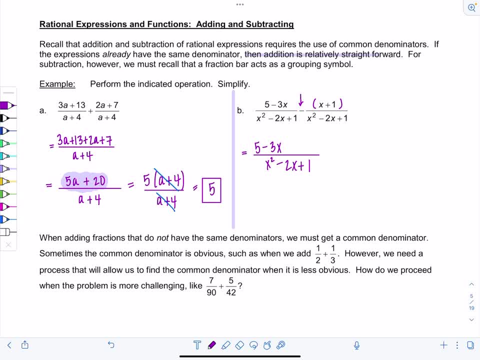 have 5 minus 3x minus x 1. Did you catch that How the negative distributes? Don't forget that. Okay, let's combine our like terms. So we've got 5 and negative 1, that's going to be 4. And then negative 3x. 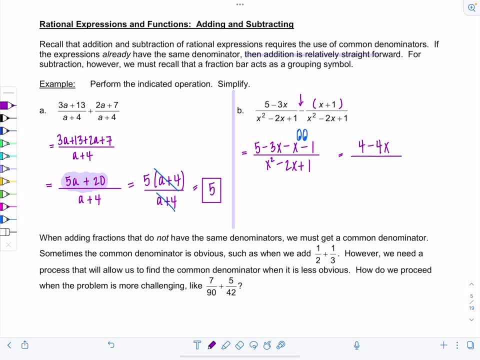 minus x, that's negative 4x over x, squared minus 2x plus 1.. All right, And no, we're not done. We have to make sure this expression is completely simplified, So let's factor the numerator, factor the denominator. If you look at the numerator, you can factor. 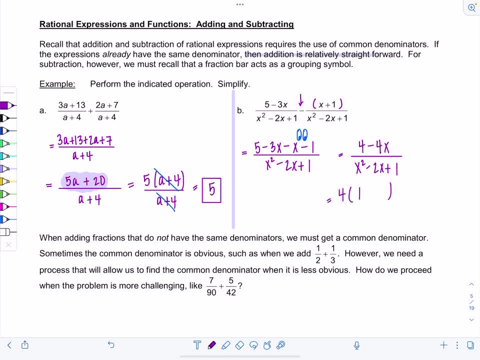 out a 4 from both terms, and we're going to be left with 1 minus x And then the denominator x squared minus 2x plus 1, that factors too. That factors into x minus 1 times x minus 1, or x minus 1 squared same thing. Do you notice anything? 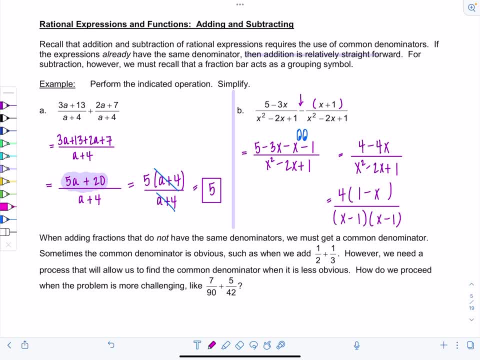 you can cancel. Remember: 1 minus x is equal to the opposite of x minus 1, since the order of subtraction is reversed. So I can cancel out. So I can cancel out these two factors, I just have to make sure I add a negative in the. 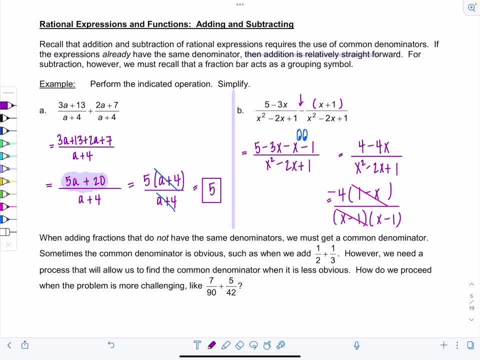 numerator And then everything is completely simplified. So we have negative 4 over x minus 1.. If you forgot about that, just review the previous video where we went over simplifying rational expressions. And whenever you add that negative, you guys, it goes in the numerator. 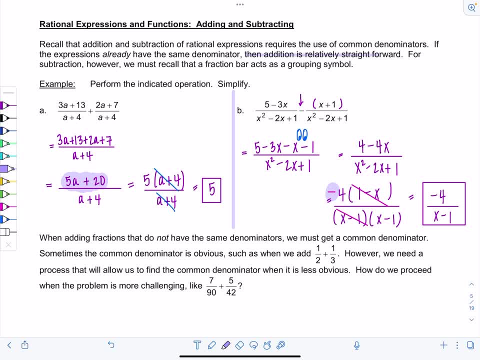 Okay, So this is not too terrible. Notice, in both examples we already had a common denominator. How nice. But life is not going to always be that easy. Most of the time you're going to run into fractions or rational expressions that don't have the same denominator, So we have to go get a common. 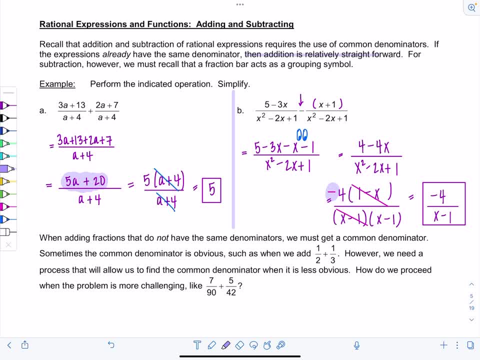 denominator And you want to use the least common denominator, not just any old common denominator, especially with rational expressions, because you don't want to have all this crazy foiling and simplifying going on in the numerator. You'll see what I mean in a second. 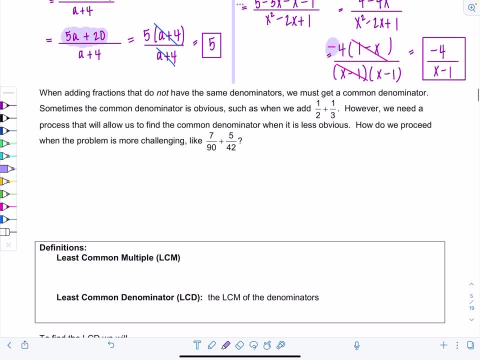 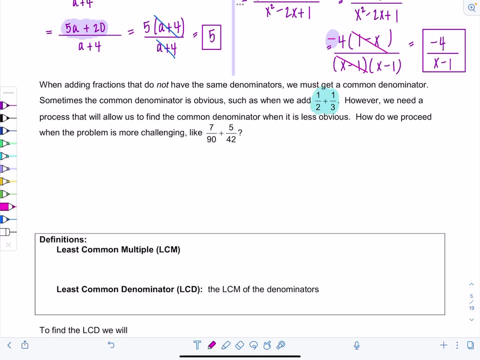 So sometimes the common denominator is pretty obvious or easy to find. If you think back, when you would add fractions like 1 half and 1 third, you could tell: okay, the common denominator is going to be 6.. And you get that just by multiplying those two denominators. 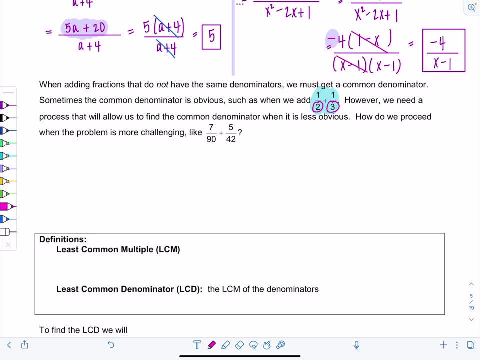 by each other. However, we need a process that's going to help us find the common denominator when it's not super obvious, like this. what do we do when the problem is more challenging, like 7 over 90 plus 5 over 42?? You don't want to. 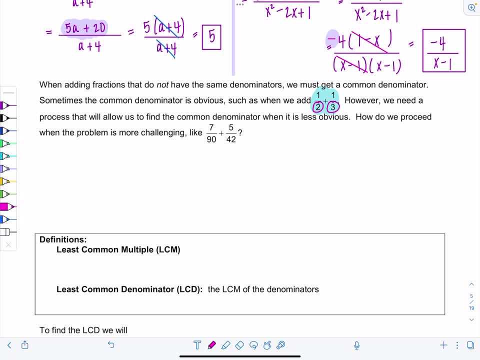 just sit there and multiply 90 and 42 by each other, because it's going to make a mess of a problem and you're going to have a wild time trying to reduce it at the end. So think back how maybe you were taught is to write out the prime factorization of each denominator. So 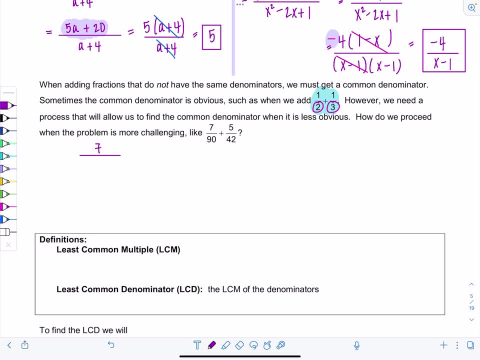 90,, that's 9 times 10, right, And 9 I can break down into 3 times 3, and then 10 is 2 times 5, and then we're adding 5 over 42.. So let's write down the prime factorization for 42.. 42 is 6. 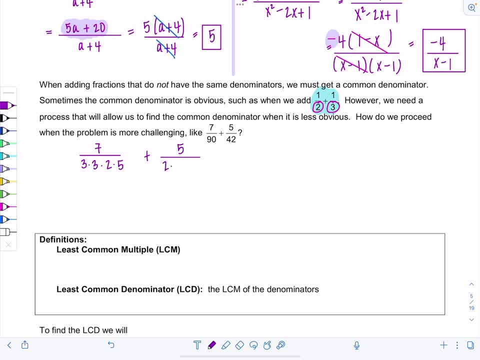 times 7, right And 6 we can break down into 2 times 3 times 7.. So what we're going to do now is build the least common denominator List, every single factor that you see in the denominator, from each fraction, one at a time. 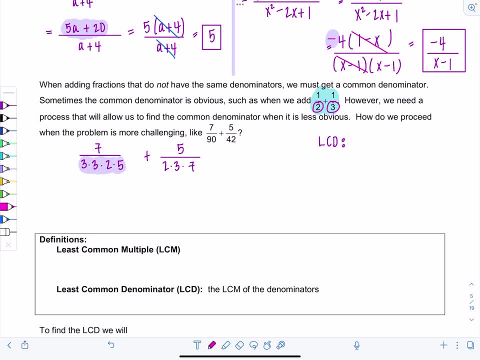 So let's see: here We've got 3 times 3 times, 2 times 5.. Okay, so those are all going to go in the LCD And then now look at your second fraction and only add in what you're missing. Okay, 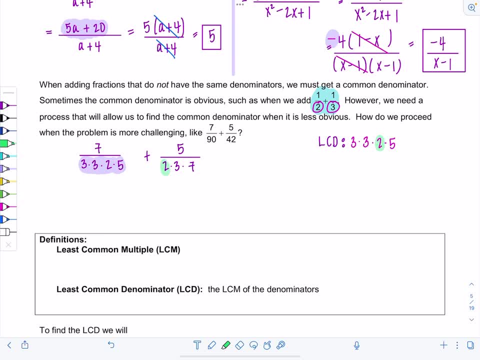 so you see this 2?? I'm not going to add another 2 because I already got it. You see this 3?? I'm not going to add it. I already got a 3.. Ooh, but what about this 7?? I don't see a 7 listed in my LCD, So I'm going to add that, Okay. 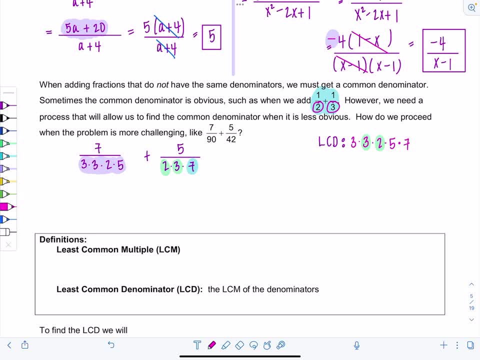 you don't add anything extra. That's why it's the least common denominator, But you do need to include all of the factors that appear in every denominator. So then, what is this LCD come out to be? This is 3 times 3 times 2 times, 5 times 7.. That's 9 times 10 times 7,, 9 times 70,. 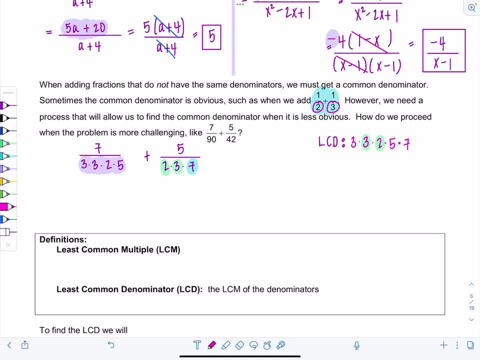 630.. If I'm doing this right, Okay, And then if you're going to add the fractions together, what would you do? Well, you compare each of the denominators with the LCD and see what they're missing. So look at this first fraction And look at its denominator. 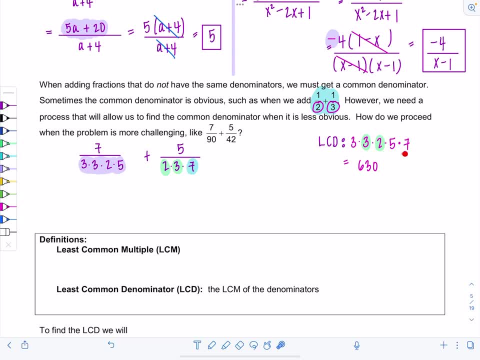 3 times 3 times 2 times 5.. It has everything the LCD has, just not the 7. So add the 7 here And here, Top and bottom, And then now look at the second fraction: It has 2 times 3 times 7.. So it has. 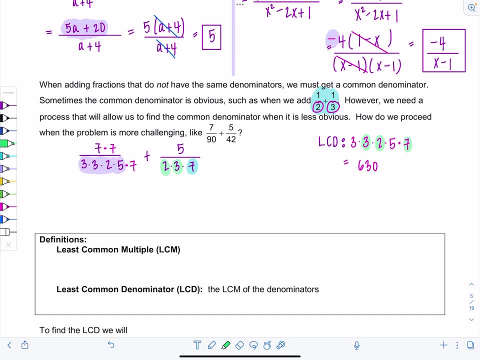 2,, 3, and 7.. It's just missing a 3 and a 5,, which is 15.. Okay, so now they both have the same denominator, which we said was 630.. So this is 49 over 630, plus 5 times 15,. 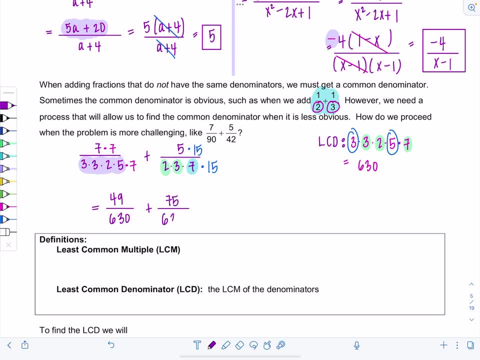 that's 75 over 630. And then when you add these together you're going to have 49 plus 75 over 630. If I add those together, that's going to be 124 over 630. And then I can reduce by 2,. 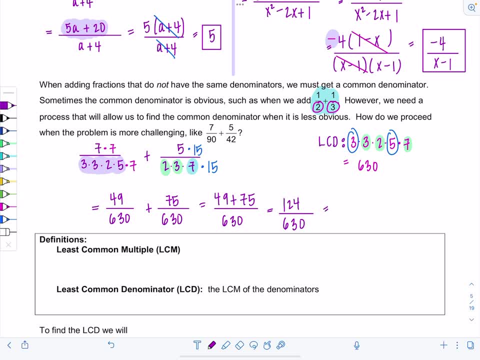 right, Cancel out of 2 from both of those. So 124 divided by 2 is 62.. And 630 divided by 2 is 315.. And now it's in lowest terms. So this is essentially the process we're going to mimic right now, just with rational expressions. 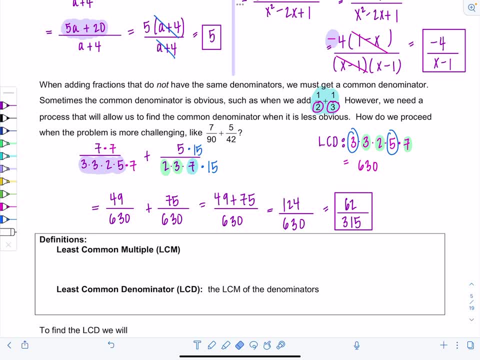 that involve variables. Okay, If you weren't taught properly how to add fractions that were more complicated like this initially in school, then it's going to be a little bit of a challenge for you. But don't worry, we're going to work through examples, building up your skill level. 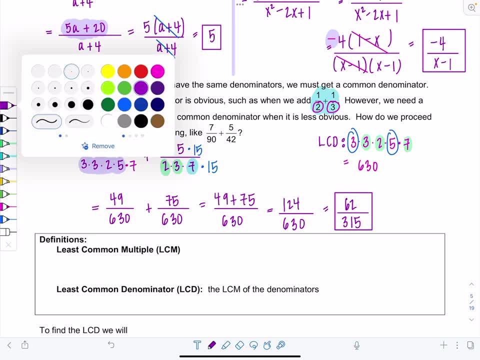 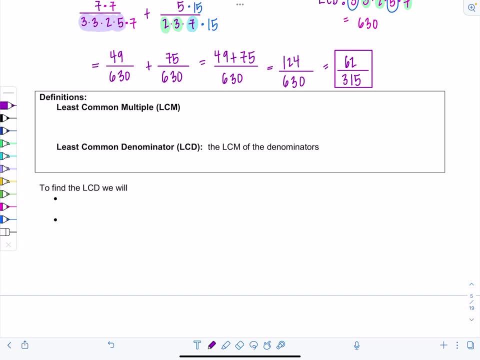 Okay, Just some definitions. Let's get them straight, because you're going to hear us using both terms a lot. So when we talk about the least common multiple, that's just a number. It's the smallest number. that is a multiple of each of the. 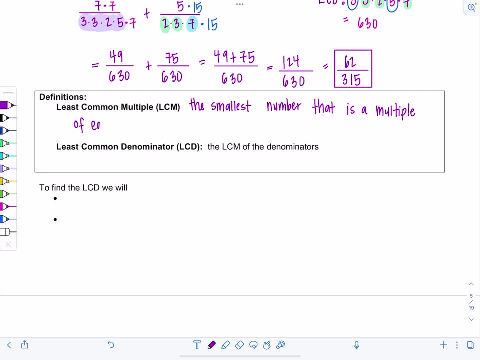 of each. And then when we talk about the least common denominator, that's the least common multiple of the denominators. So that's just being more specific, which set of numbers you're looking at? Okay, So to find the LCD, here's the steps that you're going to follow. First, you're going to 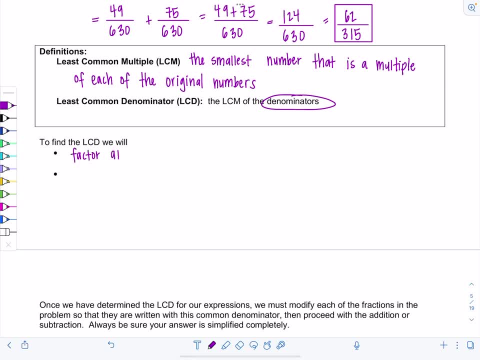 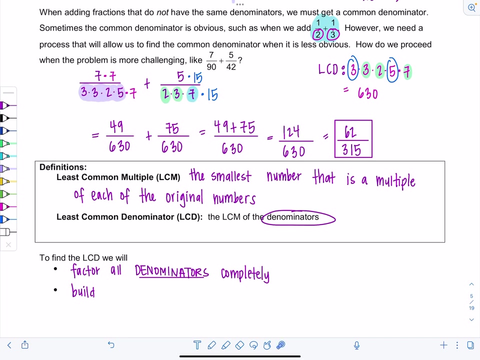 factor all of the denominators Exactly, Don't factor the numerators. Okay, This is when you're adding and subtracting. Okay, So when you're adding and subtracting, only factor the denominators first, And then you're going to build Like: do you remember how I built the LCD over here, off to the side? 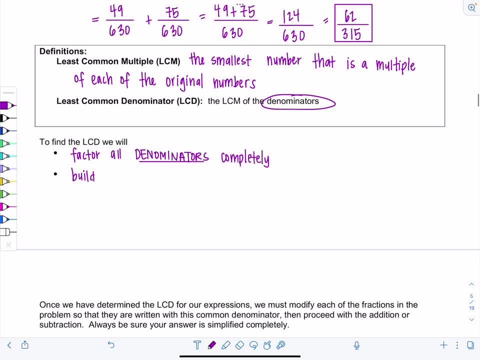 That's what you're going to do. You're going to build the smallest denominator, Okay, And then what's going to you that that'll give you is that it'll ask you to multiply the dominators, Bots As factors, Okay. 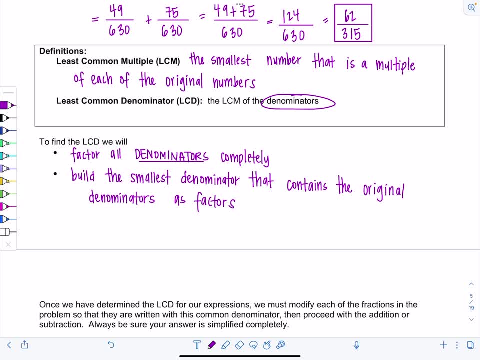 So here we go, And then, once you've determined what the LCD is for your expression, then you might a little bit more specific. And then, please- you might be wondering about the스터- modify each of the fractions in the problem So they're written with this common denominator. 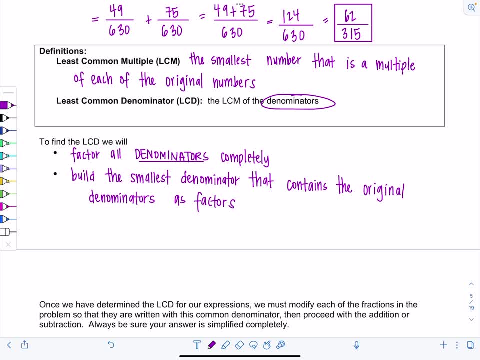 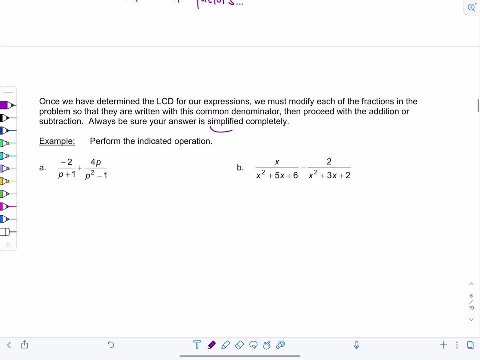 and then proceed with the addition or subtraction At the end, when you make sure that your answer is completely simplified, that's when you're going to factor the numerator and denominator. Let me use the and sign to not make you think we're adding. 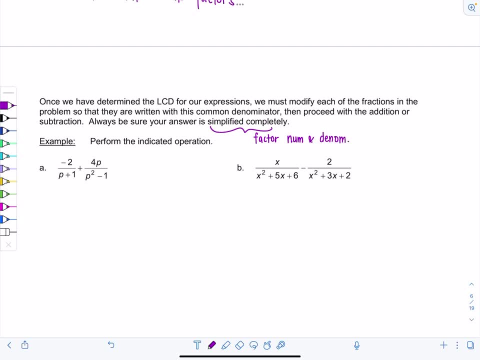 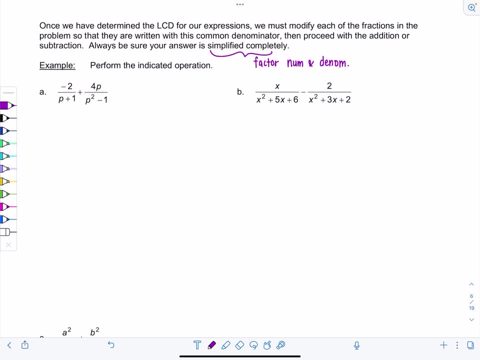 And then cancel any common factors. Okay, cool. So here we go. First example: we have negative 2 divided by p plus 1 plus 4p over p squared minus 1.. So remember, the first step is to factor all the denominators completely. So let's go ahead and do that. 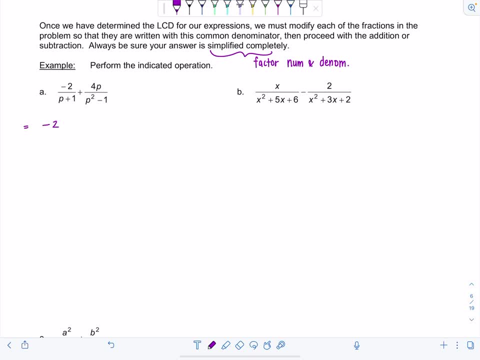 p plus 1, that's factored. So I have negative 2 over p squared minus 1.. p plus 1, leave it alone. If you want to put parentheses around it, you can, just so you know it's taken care of. Plus 4p over now. how does p squared minus 1 factor? 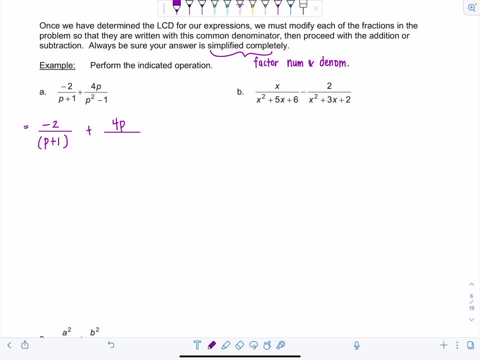 Do you remember Good? it's p plus 1 times p minus 1.. Okay, so now let's build the least common denominator. So look at the first fraction. Whatever you see has to go in the LCD. So p plus 1.. Now let's look at the second fraction. Okay, let's move this. 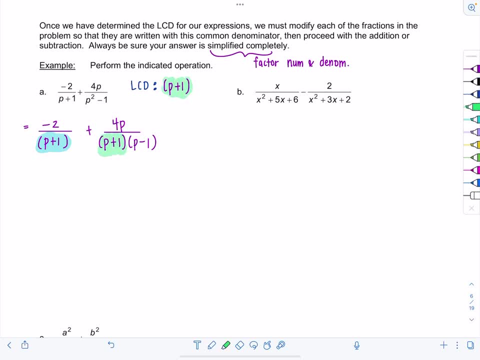 p plus 1.. Oh, I already see it in there, I don't need to add another one. This is the least common denominator. Okay, don't add excess. What about p minus 1?? Is that in my LCD? No, it's not So. 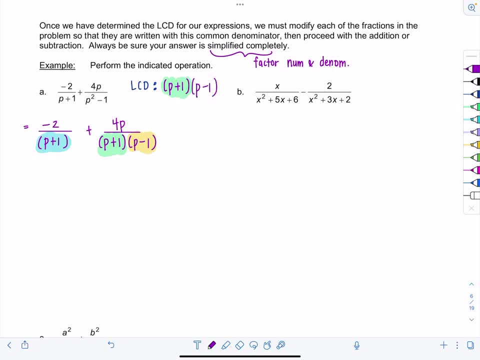 let's add it in. Okay, beautiful, Now that we have the LCD taken care of you, look at each of the fractions, each of the rational expressions. make sure they have the LCD. This guy is taken care of, right, It has the same two. 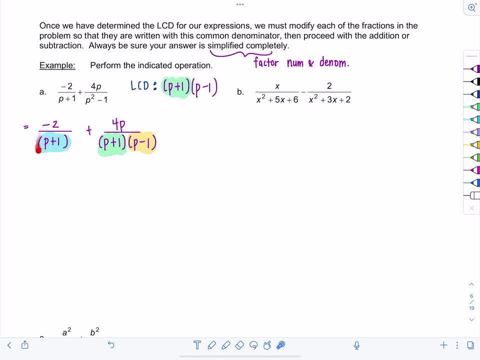 factors that I see in the LCD, Not this first little one. What's it missing? It has p plus 1, but it doesn't have p minus 1.. So I'm going to multiply numerator and denominator by p minus 1.. 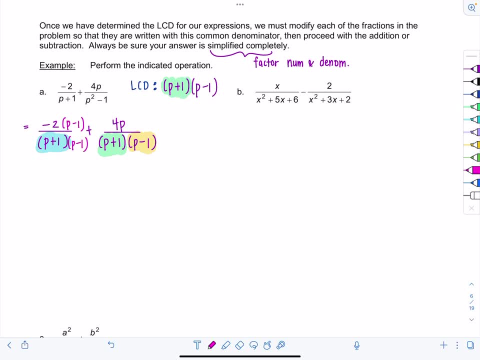 That way it has the same denominator. Okay, so now both expressions have the denominator p plus 1 times p minus 1.. So I could put everything together in the numerator. I have negative 2 times p minus 1 plus 4p. Okay, don't you even? 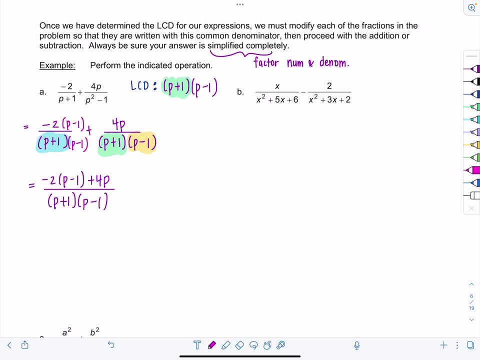 think about canceling out that p minus 1.. Illegal, illegal. We talked about it last video. We got to distribute, clean up and then refactor. So this is the denominator. I have negative 2 times p minus 1.. 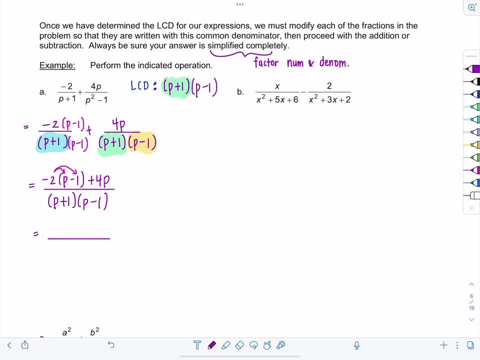 Okay, so now both expressions have the denominator p plus 1 times p minus 1.. So I could put everything together over here. So I have negative 2 times p minus 1.. Let's see Negative 2p plus 2. 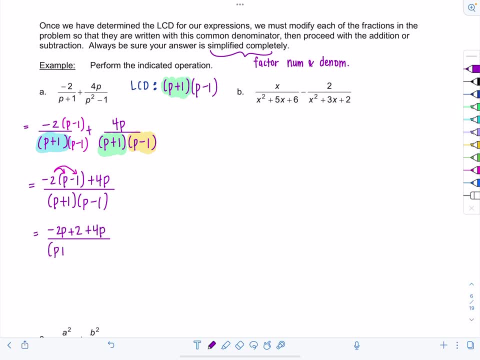 plus 4p and then leave this denominator factored: P plus 1,, p minus 1, and then let's see, here Can we combine some like terms in the numerator: Yes, Negative 2p plus 4p, That gives me 2p. Then 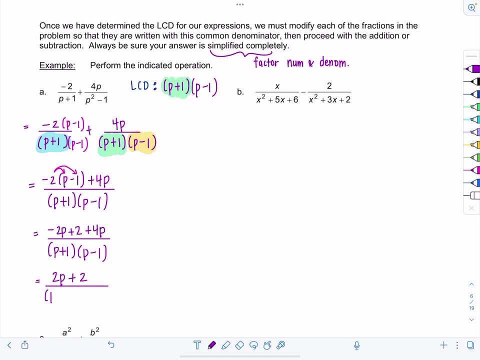 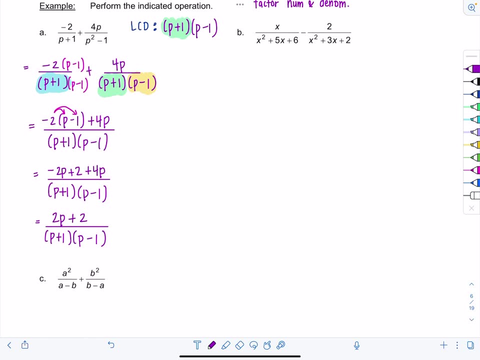 I have plus 2 over p, plus 1 times p, p minus 1.. Nice, And then can we factor the numerator- Yes, we can take a 2 out, And then I have p plus 1 left over p, plus 1 times p minus 1.. 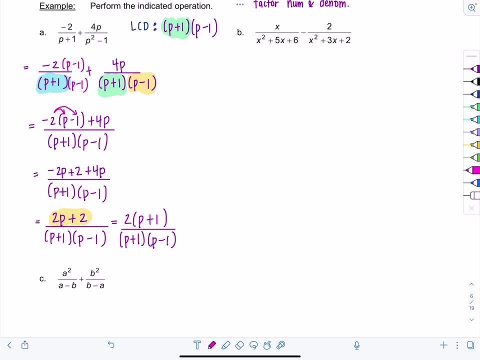 And then, last step, we can cancel out p plus 1, and our final answer is going to be 2 over p minus 1.. Okay, So sometimes it's difficult because some of the rules of mathematics- especially when you're 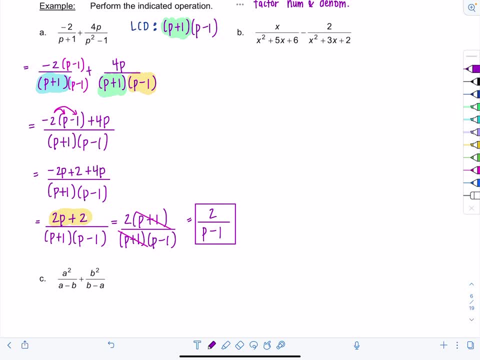 first learning them won't feel natural. You're going to have to keep reminding yourself what you are and aren't going to be doing. So I'm going to keep reminding you that. So I'm going to keep reminding myself what you are and aren't allowed to do. But the more you practice and take your 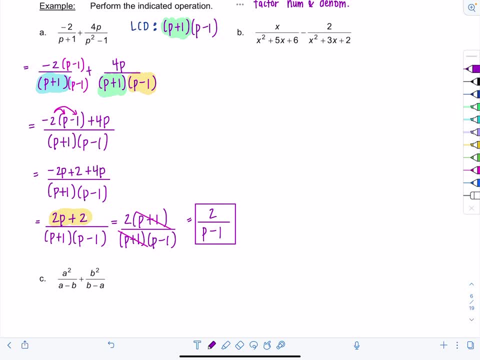 time it will come to be more second nature to you. You won't have to stop and think just like when you learn a language. Maybe you haven't gotten to the point where you've learned a language and become fluent, but it can be possible. One day you will stop conjugating and you'll just speak. 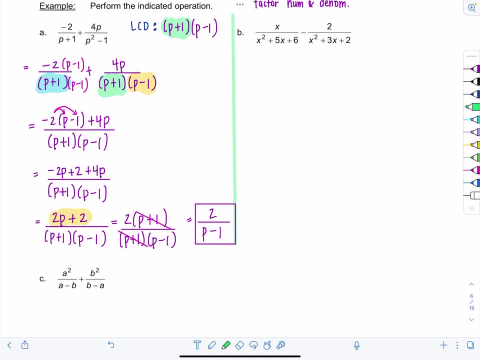 properly. Okay, Let's look at example B To start off. we want to factor all those denominators, Okay, So let's do it. We've got x over. how does x squared plus 5x plus 6 factor? 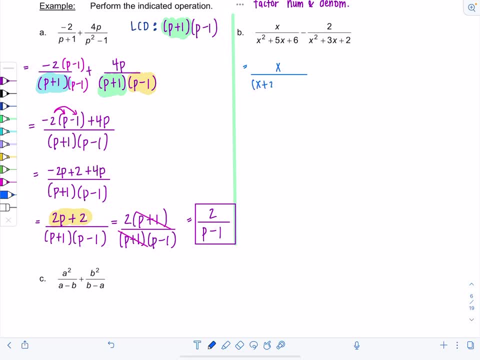 Be careful with this one. Yeah, It's x plus 2 times x plus 3 minus 2 over. how does x squared plus 3x plus 2 factor? Very good, x plus 1 times x plus 2.. All right, Let's see if we can build the LCD now. 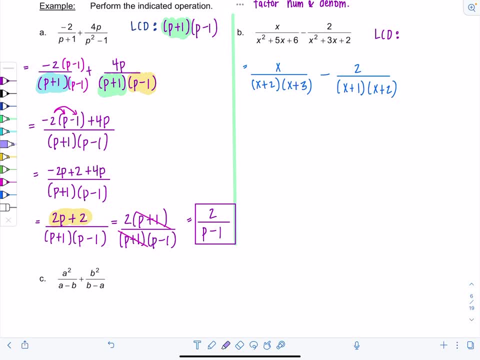 So look at the first fraction. Its denominator has the factors x plus 2 and x plus 3.. So those have to go in the LCD. Now I'm looking at my second fraction, or rational expression: x plus 1.. I don't see that there, So let's add that in. Do I need to add in x plus 2? No, 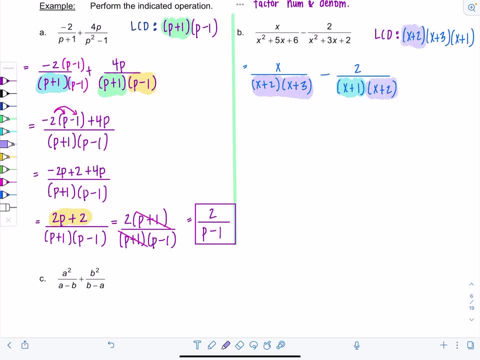 because I already see x plus 2 taken care of. So we are good, All right, Don't overkill, Don't overload the LCD, then it won't be the least common denominator. Okay, Now let's make sure each of these denominators is the LCD. So first one, first rational expression. 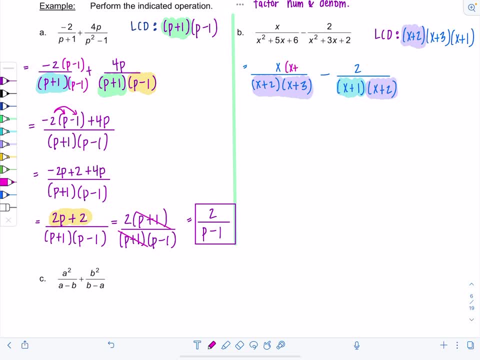 has x plus 2, x plus 3.. It's missing x plus 1.. So we'll multiply that in the top and bottom. All right, one is missing: x plus 3.. Good, Okay, so now we can put everything over the same denominator. 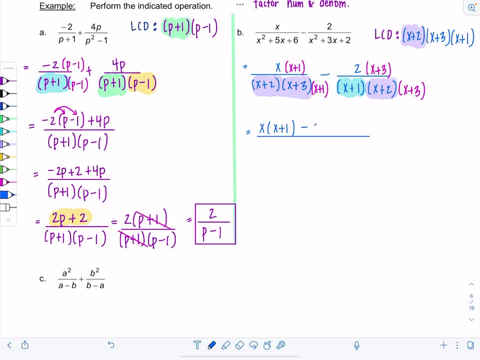 We have x times x plus 1 minus 2 times x plus 3 over x plus 2, x plus 3, x plus 1.. Okay, no canceling yet I'm going to say it over and over. You see how there's subtraction here. 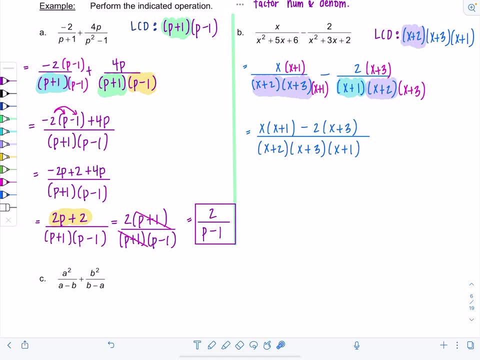 That means it's not time to throw your cancel party. You have to finish distributing, cleaning up, refactoring at the end. then maybe it's cancel party time. You see how the denominator is fully factored. It's just bam, bam, bam, factor, factor, factor. The numerator has to. 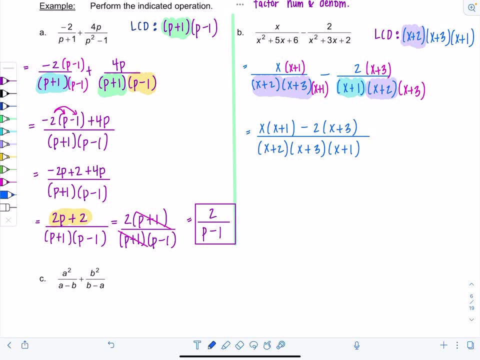 be the same way in order for you to be able to cancel. Okay, so let's distribute x times x plus 1, that's going to be x squared plus x minus 2x minus 6, over x plus 2, x plus 3,. 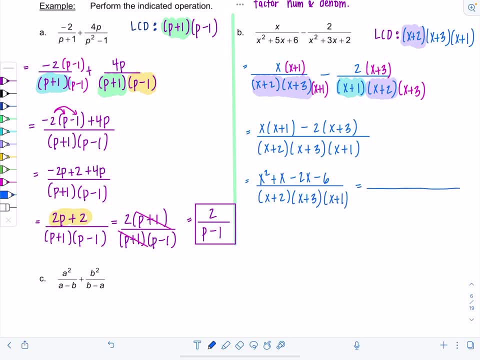 x plus 1.. Can we combine like terms: Yeah x and negative 2x, So we have x squared minus x minus 6 over x plus 2, x plus 3, x plus 1.. Almost there Does this work. 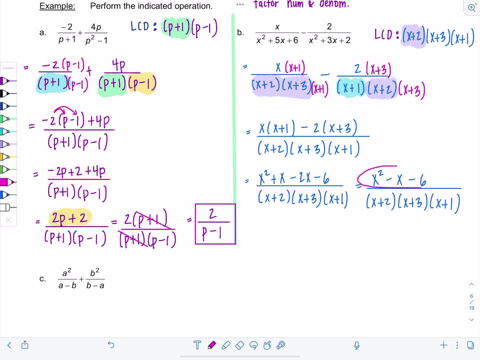 The numerator factor x squared minus x minus 6.. Does that factor? It sure does. It factors into x minus 3 times x plus 2.. Okay, so let's see. Is there anything that we can cancel? We can cancel x plus 2.. 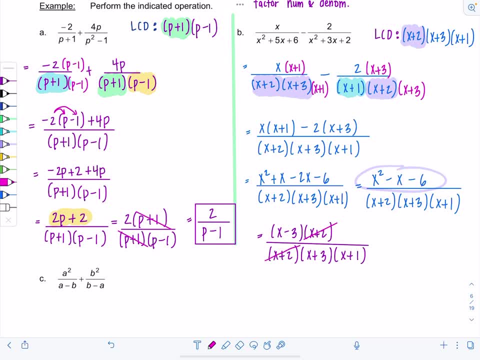 Okay, so let's see. I see that same exact factor in the numerator and denominator, x plus 3 and x minus 3 are not the same. You can't cancel. when one factor has addition, one has subtraction. No, no, no, So that's it. That's as much of a party as we're going to have. 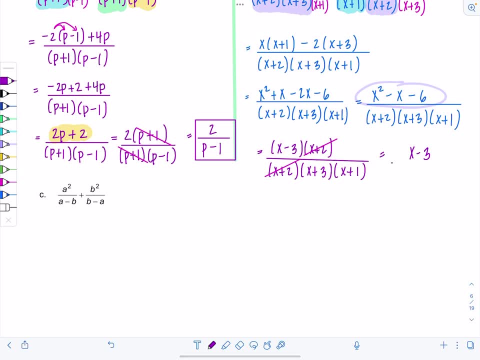 with this problem. So we've got x minus 3 over x plus 3 times x plus 1.. Lovely, Okay, that was fun, Okay. next example: Example C: a squared over a minus b plus b squared over b minus a. 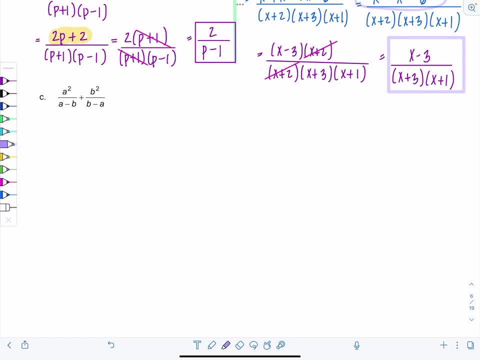 Okay, here's a cool little trick. Whenever you're trying to add or if you're subtracting rational expressions and you notice the denominators are identical, it's just the order of subtraction is reversed. It's usually best to switch the order of subtraction in the second expression. 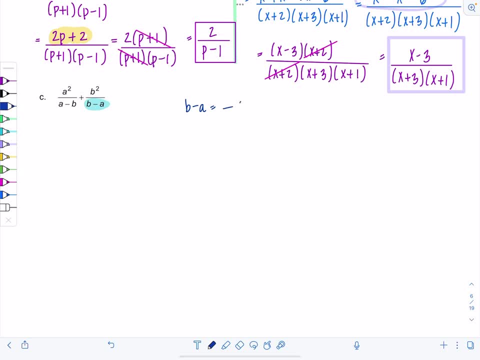 And remember: b minus a is equal to the opposite of a minus b, So I can replace b minus a with a minus b. I'm just going to have to add a negative. Where do I add it? You should always add it in the numerator. 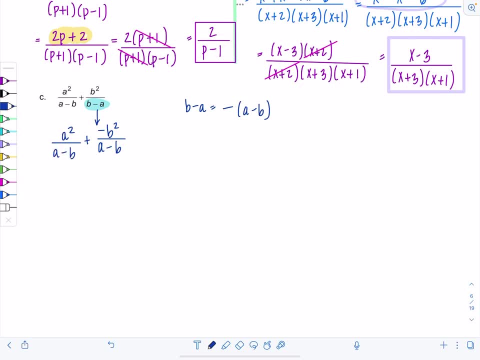 So now I have a squared over a minus b, plus b squared over b minus a, or basically this is the same thing as just doing a squared minus b squared now over a minus b. so sometimes my students like to just use the shortcut where they switch the. 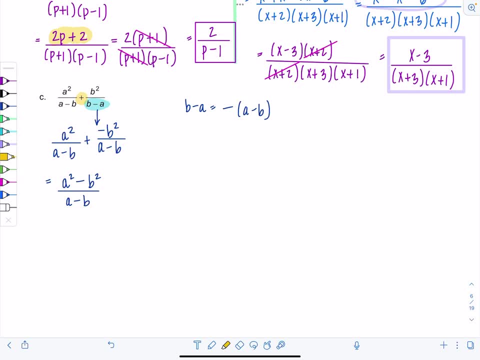 addition to subtraction, and then rewrite the second denominator to match the first one, and if originally it was subtraction, then you would switch it to addition. right, because the two negatives would cancel out and make it positive. okay, not too bad. huh, that little shortcut really saved time. um, can we factor anything? yes, a squared minus b squared, that's. 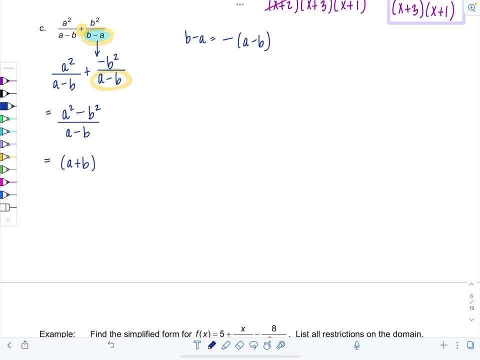 difference of square. so that's going to factor into a plus b times a minus b over a minus b. now go ahead, you can cancel a minus b. that means there's just a one in the denominator and you don't have to write it in your final answer. so we're just left with a plus b. very good, okay, are you feeling a little? 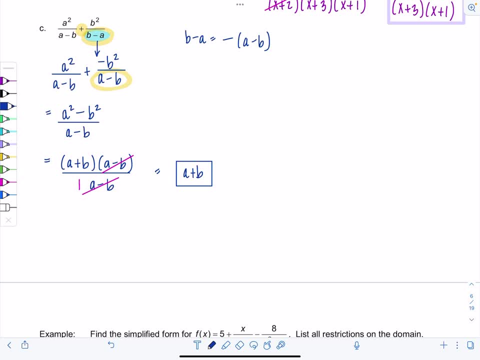 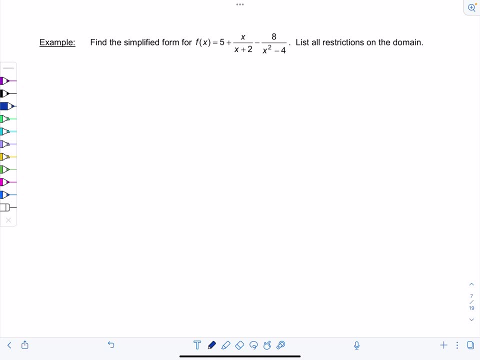 more comfortable? I hope so, okay, last example: find the simplified form for the following function: f of x equals 5 plus x over x plus 2 minus 8 over x squared minus 4, and list all restrictions on the domain. so I'm going to rewrite this and I'm going to do it again. so I'm going to do it again and I'm. 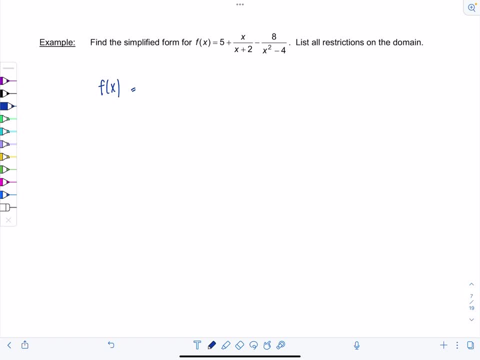 gonna write f of x, factoring all the denominators, and I'm going to put 5 over 1, because that's what its denominator is. we just don't normally write it, but it'll help us when we try to find the lcd and make sure everything has a common denominator. okay, plus x over x plus 2 minus 8 over and then: 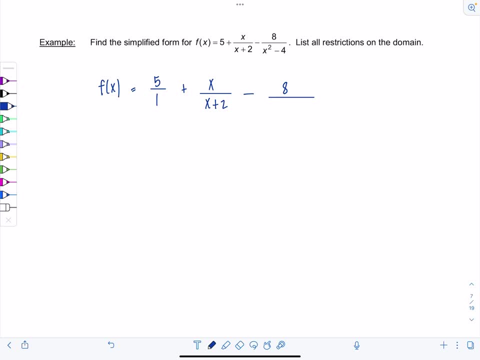 factor. please. what do you get? good good x plus 2 times x minus 2.. All right, let's list all the restrictions on the domain here. Well, it's really easy to see. So you want to restrict any values of x that would make the denominator 0.. 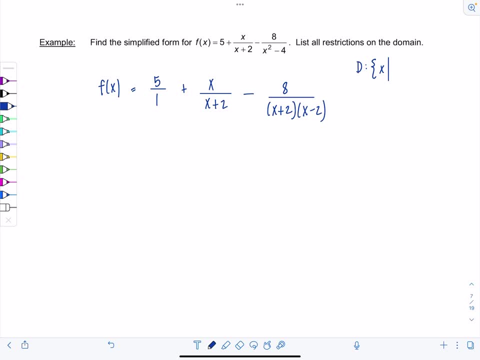 So we say: the domain is all x's, such that that's how you read that vertical line x does not equal. Okay, there's no variables here, so I have no restrictions Here. I can see: x cannot equal negative 2. Why I wrote it backwards that way, I don't know. And then here we see again: x cannot. 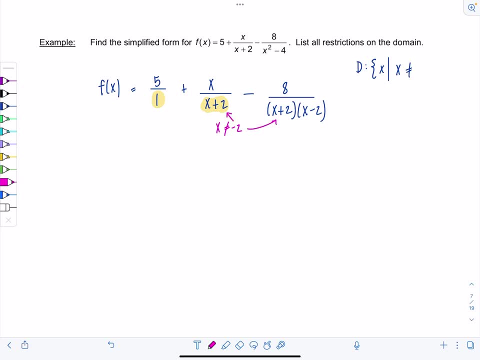 equal negative 2, that popped up in two places- and also x cannot equal positive 2.. So you can actually list both those restrictions together. x cannot equal plus or minus 2.. That's the domain. Okay, now let's go ahead and figure out the LCD. 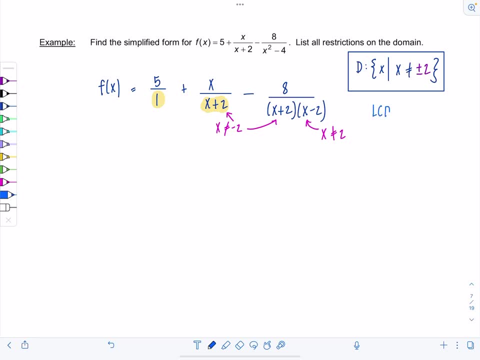 least common denominator. Did you do it already? 1 is in there, who cares? x plus 2.. And then notice here: okay, we already have x plus 2 in the LCD, so just add x minus 2 to it. Good, Very good, Now we have. 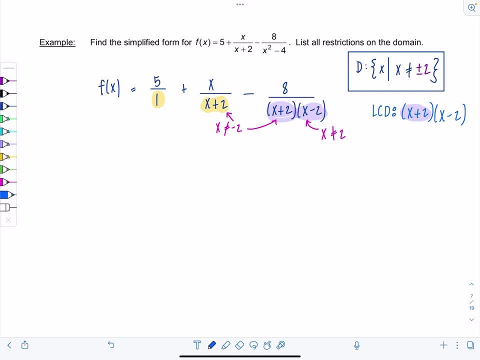 to make sure each of the terms has the LCD. So 5,. this guy's missing everything. It needs both x plus 2 and x minus 2.. Top and bottom. The second term only needs x minus 2, and the last term needs nothing. okay. 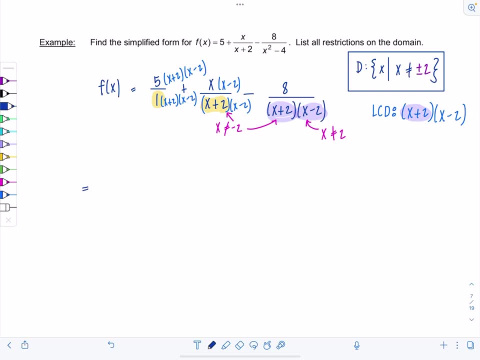 So let's put everything together over the same denominator, which is x plus 2 times x minus 2.. So I have 5 times x plus 2, x minus 2, plus x times x minus 2, minus 2 minus 8. now I'm taking this really step by step, if you already can. 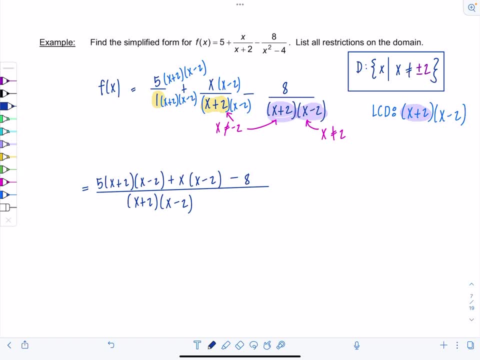 start multiplying stuff out, go for it. okay, when you take 5 times X plus 2, X minus 2, anytime, you just have one little term and then you're multiplying it by two other factors that involve addition or subtraction. multiply those guys out first and then multiply by the 5 last. okay, bring that little loaner in at the 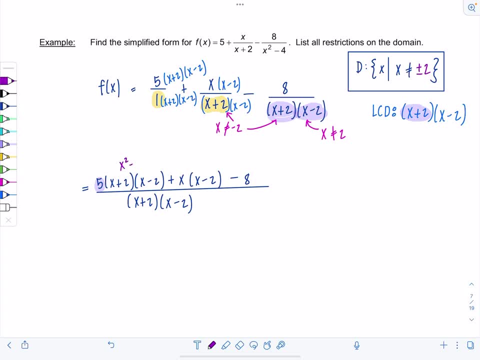 very end. X plus two times X minus two is in that X squared minus 4, and then you're gonna multiply that by five, right okay? so then we're gonna have 5 X squared minus 20 plus and then distribute this cute little X X squared. 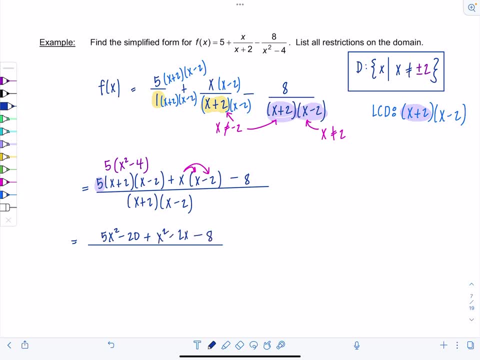 minus 2x and then minus 8. leave the denominator factored because, remember, we're gonna check if we can move our results can cancel anything out at the very end. Okay, good, So let's see 5x squared. I can add that: 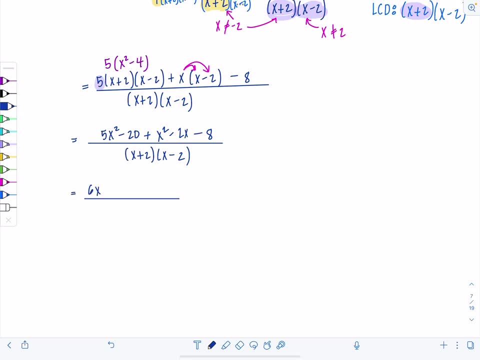 to the 1x squared and have 6x squared, And then minus 2x, negative 20 minus 8, that's negative 28. And then we have x plus 2, x minus 2.. Okay, so, let's see, can we factor this numerator? 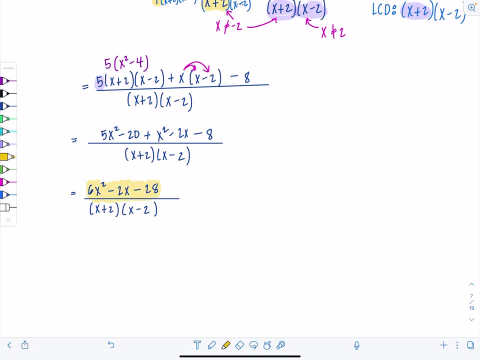 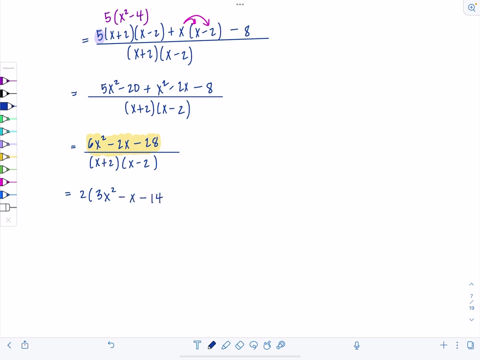 Always take out the GCF greatest common factor first before you try to. you know, break up that trinomial And I notice I can take a 2 out of everything. So I'm going to write that 2 out front. And then we have 3x squared minus x minus 14 over. that is a crooked fraction bar. 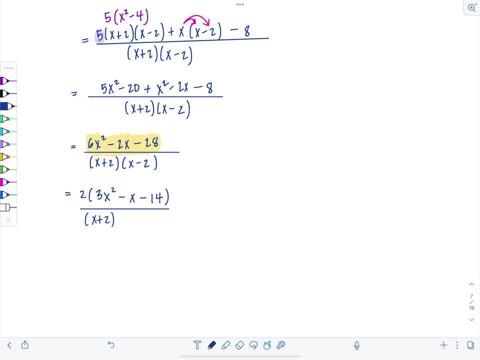 let me straighten it up. There we go: x plus 2 times x minus 2. So 3x squared minus x minus 14. How's that going to factor? If you need a refresher on factoring trinomials, 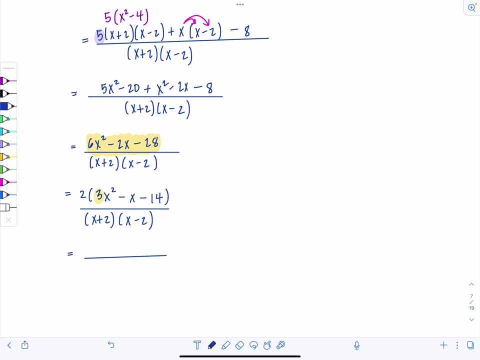 where this lead coefficient isn't 1, I'll link a video here. It's pretty quick. I like to live on the edge. I just do guess and check. That's what they taught me when I was in school. There was no method, or at least my teachers didn't know one. So let's see 14.. 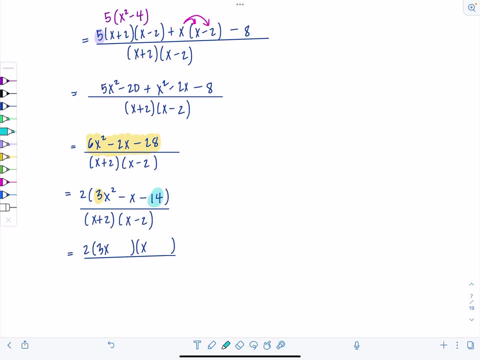 Here's what works: 14 is either 14 times 1, or 7 times 2.. Like 95% of the time, pick the two factors that are closer together, Meaning don't pick 14 and 1, unless you notice that, like, this number in front of x is really big. It's just. 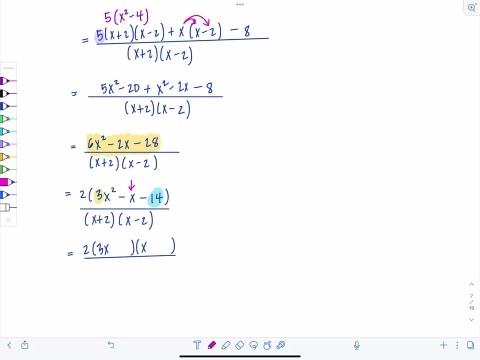 negative 1, which is not, So I'm going to go with 7 and 2, instead of 14 and 1.. And then play around with it Like I'm. I don't want the 7 here, because that's going to give me 21x. What the. 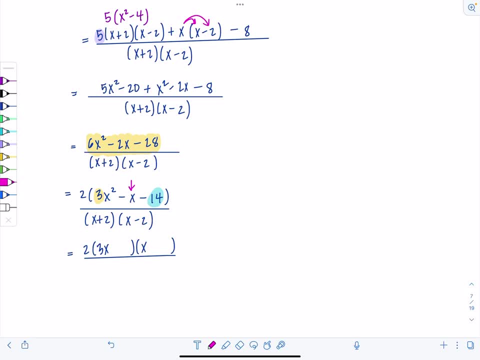 heck, How would I get a negative 1 in front of the x? No way, no, how. So I'm thinking we're going to put the 7 here, the 2. Here, and then bam, I can already see: this is plus, this is minus, because this would give me. 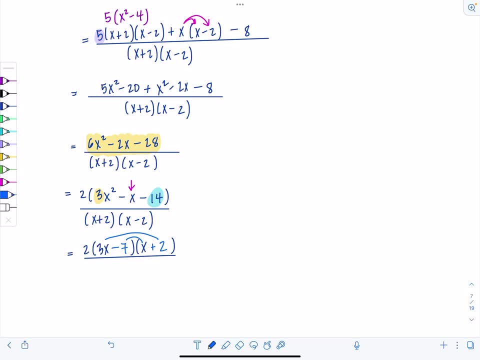 positive 6x, negative 7x, And I just do all that in my head pretty quickly at this point. okay, And then denominator is still x plus 2 times x minus 2.. If you hate guess and check, though if it just makes you too nervous, then do the method that I show you in that video that I